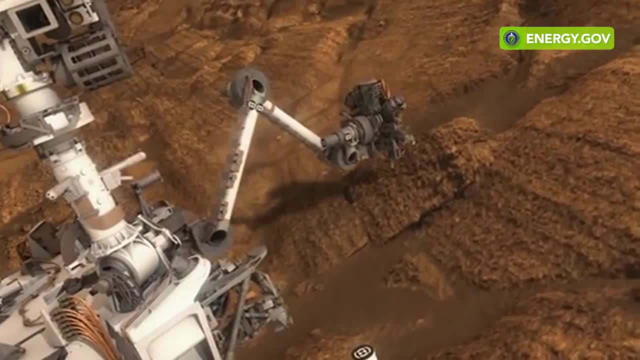 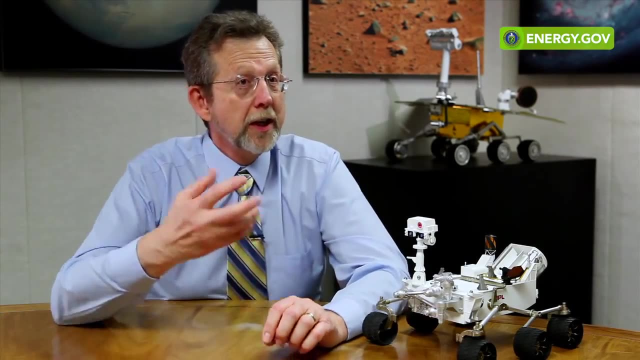 to generate electricity which can be used by a spacecraft. That's important because it enables us then to run experiments. charge batteries survive the night. We can use the heat from these systems to keep everything at a particular temperature that allows it to survive. 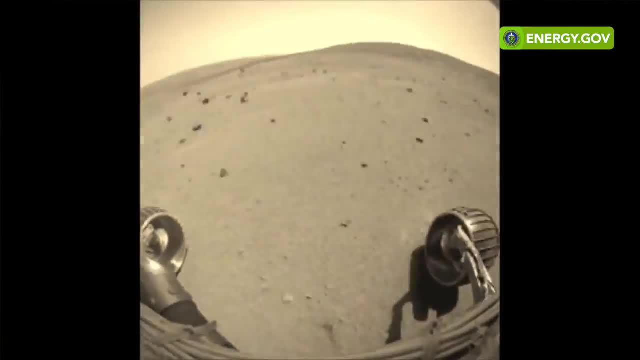 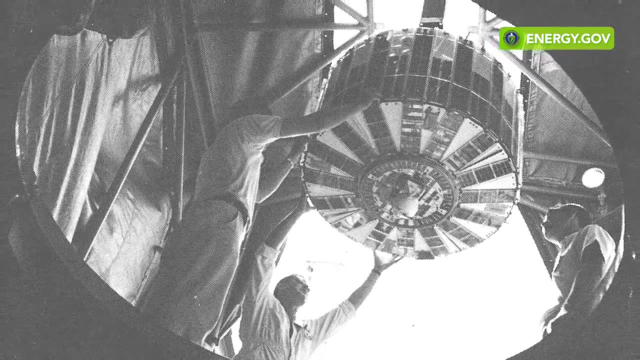 And because of that, then, it enables us to operate in space. There are certain missions that we could have never done using traditional solar power. The first nuclear-powered satellite was launched in 1961. It was the Navy's Transit 4A satellite. 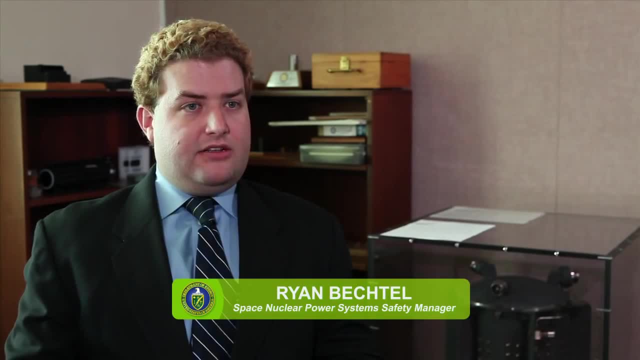 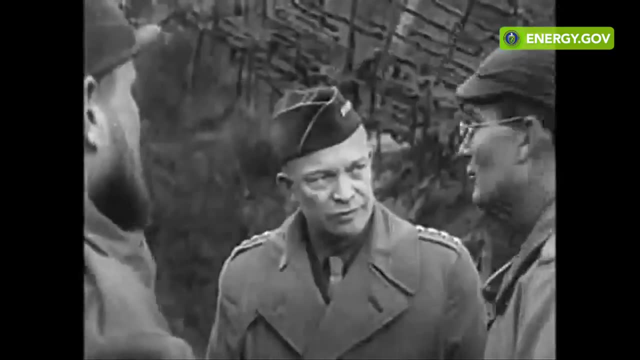 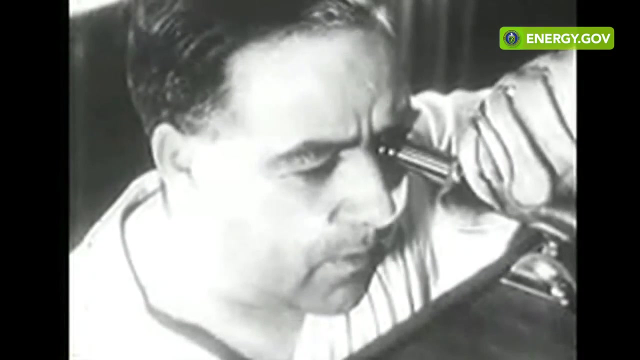 It was used by the Navy as a predecessor to today's Global Positioning System satellite network. They were first developed under the Atoms for Peace Initiative under President Eisenhower. First. encourage worldwide investigation into the most effective peacetime uses of fissionable material. 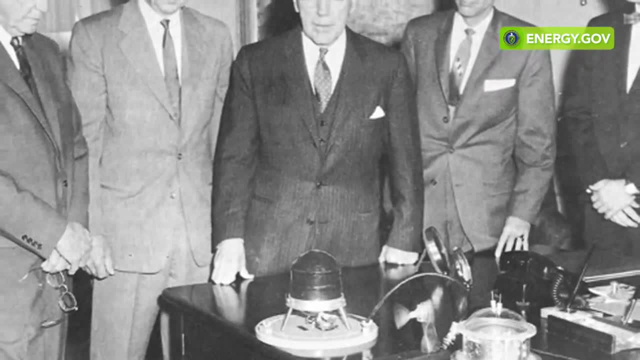 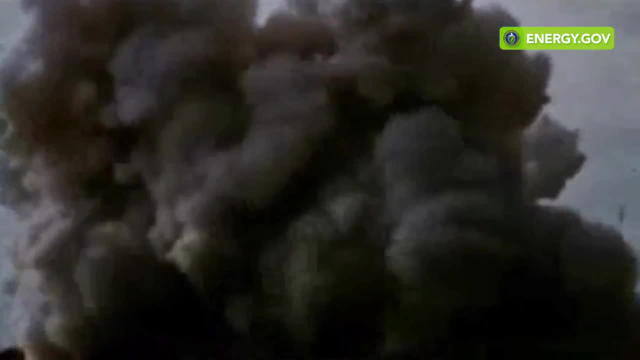 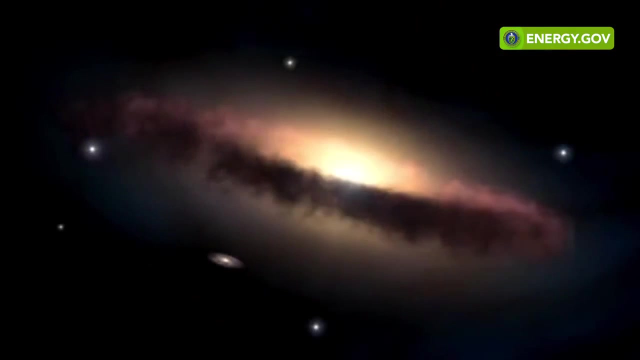 And the first public introduction to a radioisotope thermoelectric generator was in President Eisenhower's Oval Office. Since then, we've launched over 27 missions using nuclear power systems in outer space. So then NASA began using RTGs to enable their deep space exploration for about a decade. 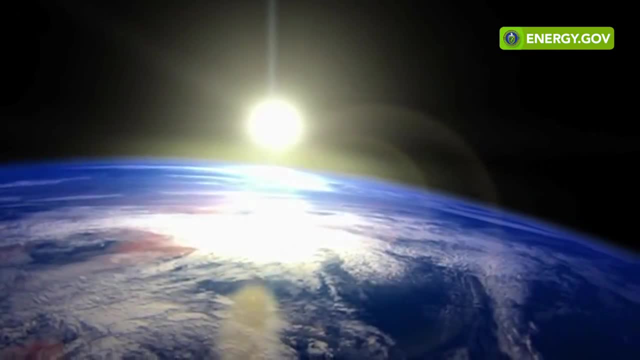 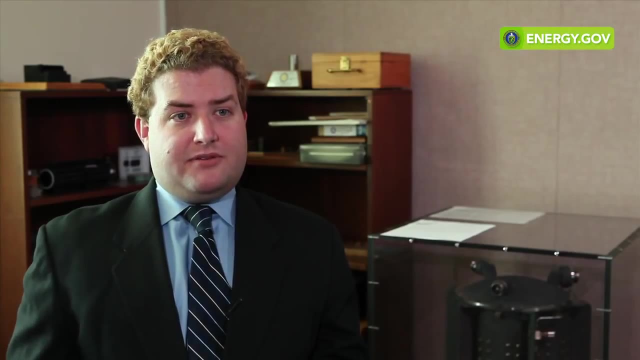 And during this time there were some changes. back here on Earth, The Energy Research Development Agency became the Department of Energy And since then the Department of Energy with NASA have teamed up to produce long-lasting, reliable power systems for deep space exploration. 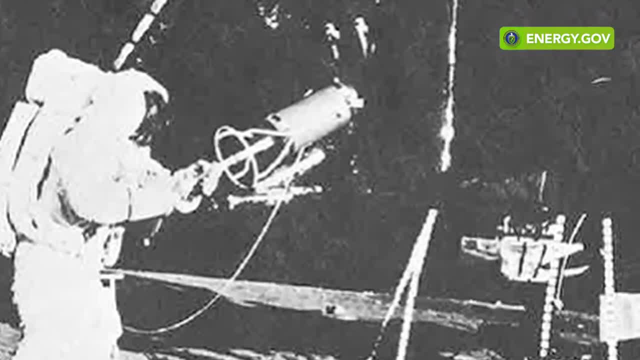 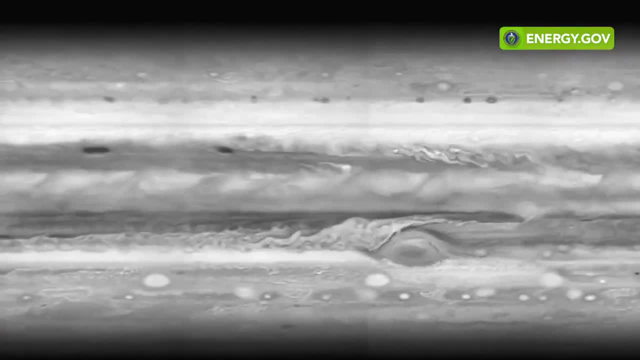 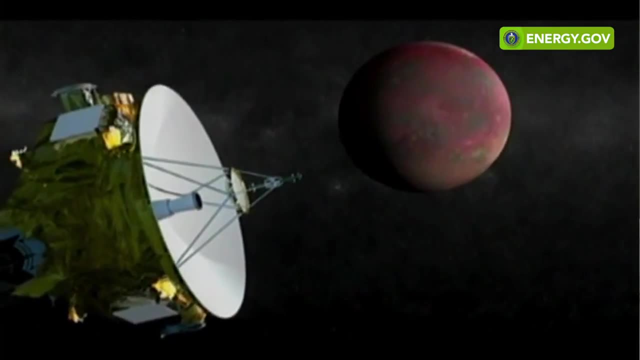 We've had generators on the Moon. They've done flybys of Venus, Uranus and Neptune. The Galileo mission to Jupiter. We're currently orbiting Saturn with the Cassini spacecraft New Horizons going to Pluto. We're supposed to arrive there about. 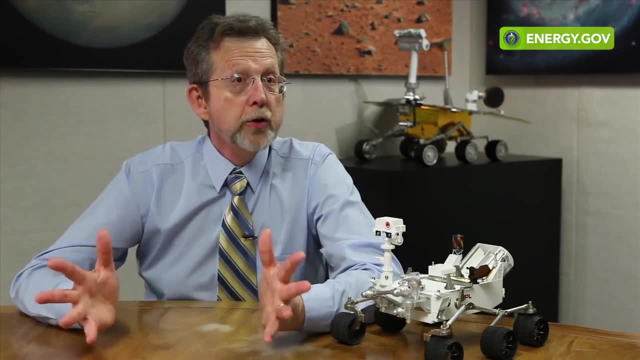 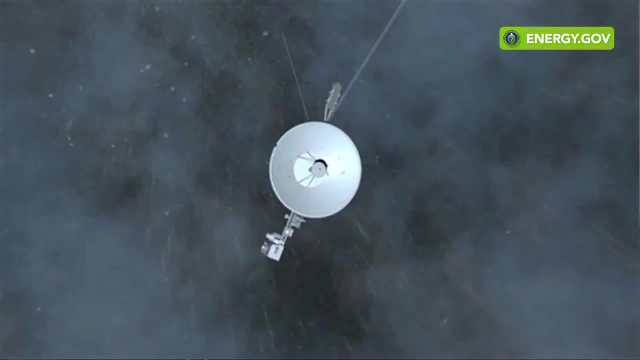 2015.. And then there's the Voyagers 1 and 2.. The Voyager space probes, launched in 1977, are still operating today because of their radioisotope thermoelectric generators. The space probes are over 11 billion miles from Earth. 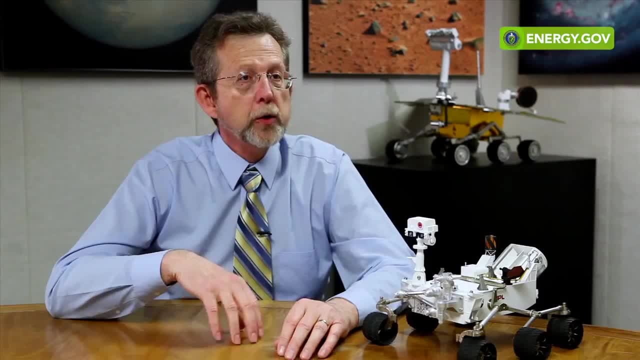 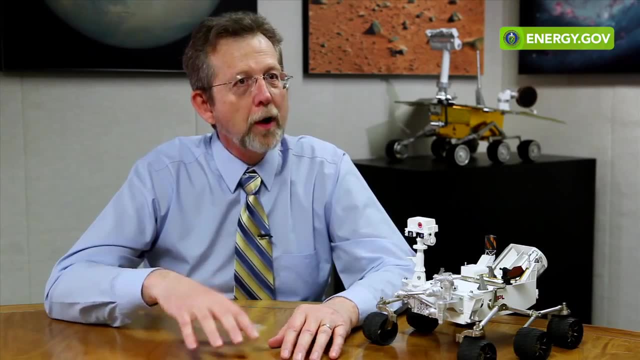 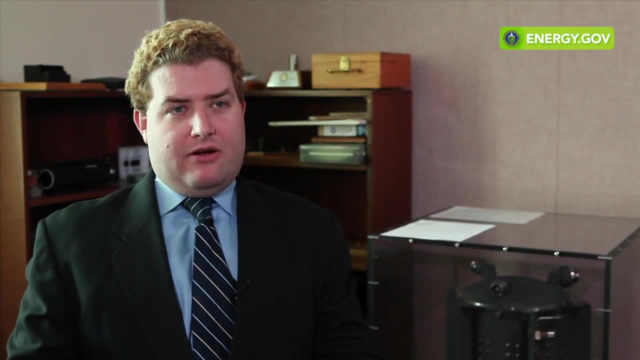 and are entering the very fringes of our solar system. As we look at these objects and study them, we really determine that there are places in the solar system where life might actually exist well beyond the boundaries of our Earth. Radioisotope power systems enable our understanding of the outer solar system.